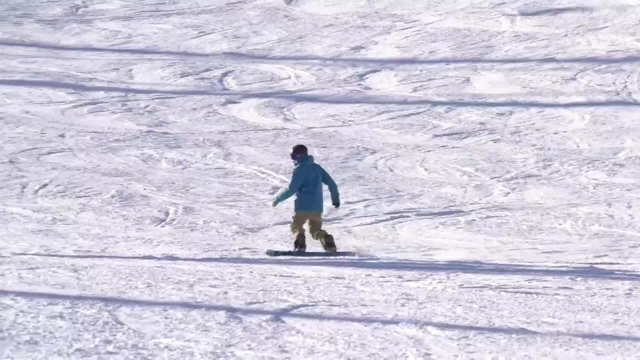 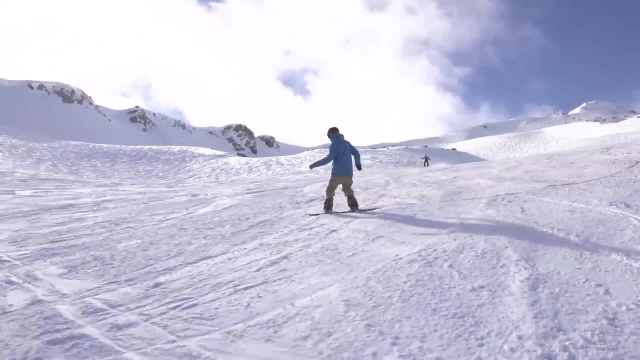 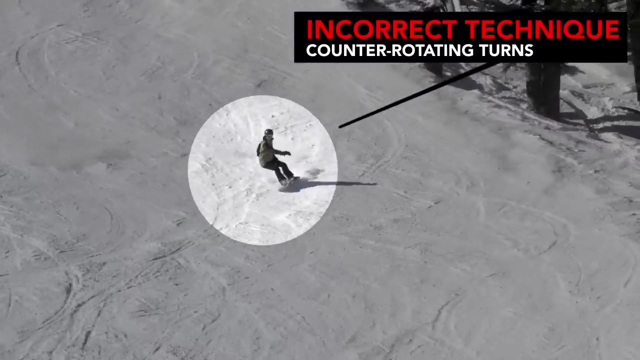 For smooth, controlled riding, you want your upper body and lower body to be in line with one another, because it gives you better balance and stability over your snowboard. One of the most common problems for intermediate riders is riding with a body position that is not aligned. I see a lot of snowboarders. 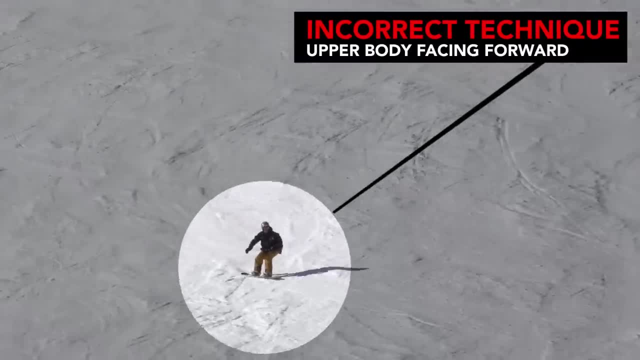 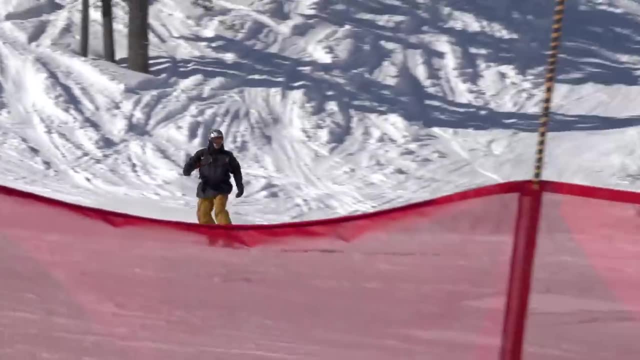 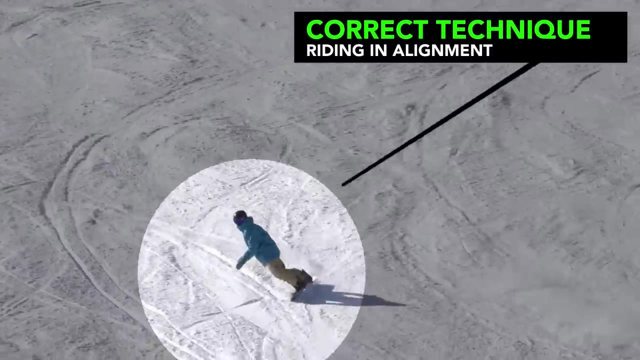 cruising with the upper body turned in this position facing forwards. It's not very stable. If you hit a bump, it's likely you'll get thrown off balance and may crash. Instead, you want to be like this, with your upper body and lower body are in line with your board. An aligned body will give you the strongest balance. 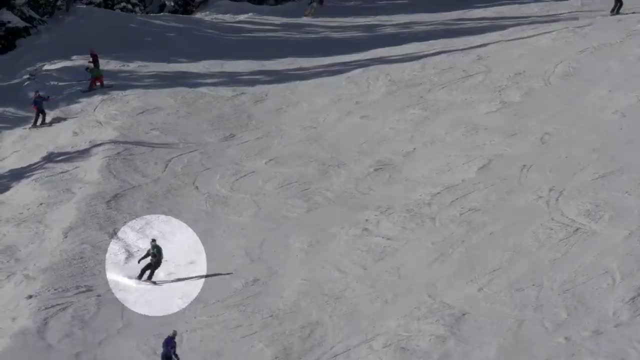 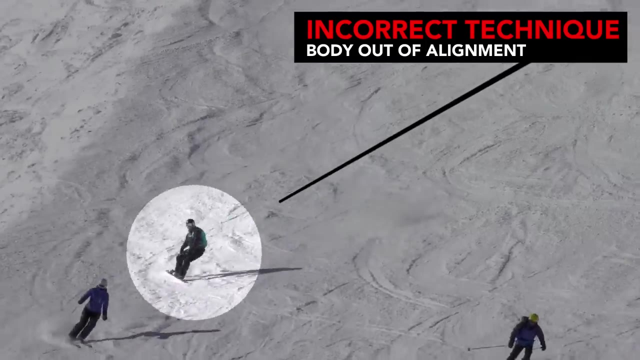 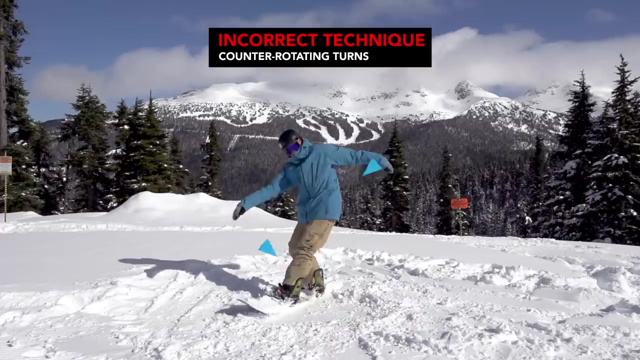 over your board. It's common to see riders going down the mountain with forced turns, constantly riding out of alignment and lots of arm swinging. This is called counter rotation, where your upper body and lower body become disjointed, not working in harmony and twisting against each other to make 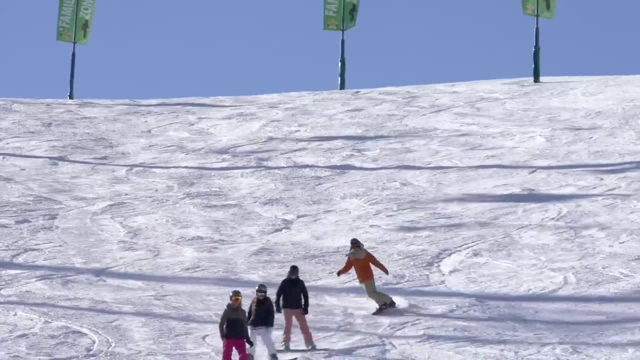 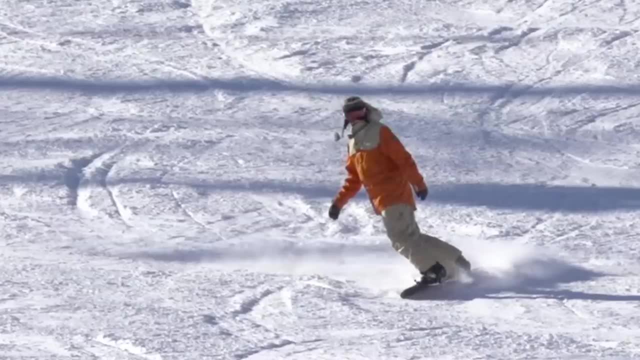 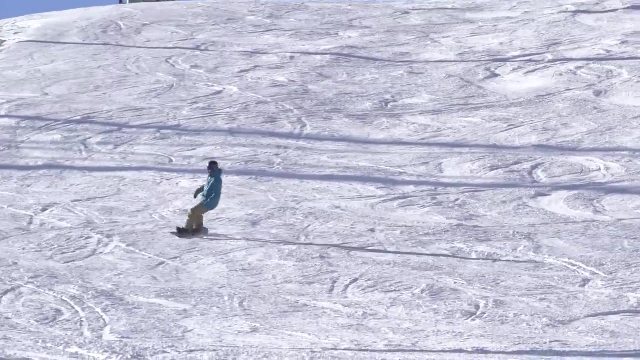 turns happen. This especially happens when doing turns on your toe edge On this freeze frame. you can see how the rider's upper body is completely out of alignment with the lower body. If you compare this with my riding, you'll see that every time I make a turn, my upper body and lower body are almost always. 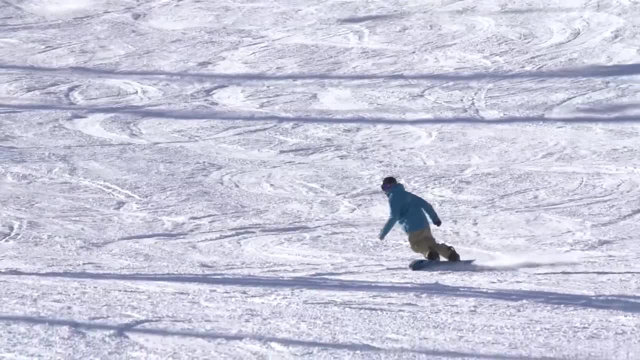 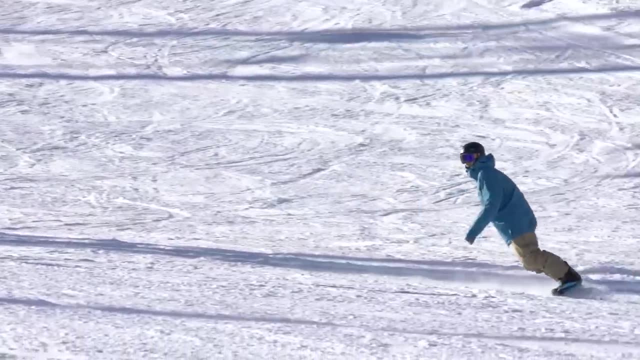 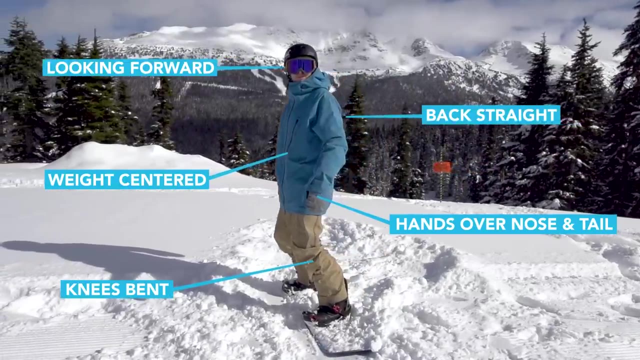 turning in the same direction. It looks smooth, balanced and effortless as I flow through each turn. If you can get your riding to look like this, then you'll be comfortable riding faster and learning new tricks On flat ground. this is what good alignment looks like. When I do a toe edge turn, you'll see my upper body. 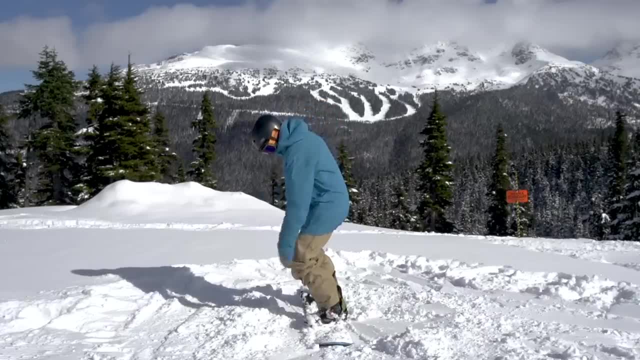 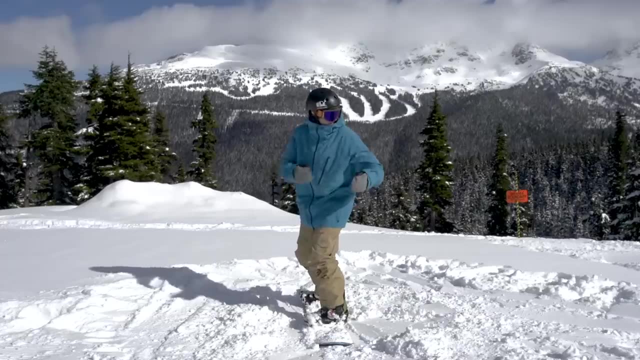 helps initiate the turn. My leading shoulder, my hip, my knee all go in the same direction. On a heel edge turn, my upper body turns, my hip turns, my knees turn, all in the same direction. You probably don't know whether you 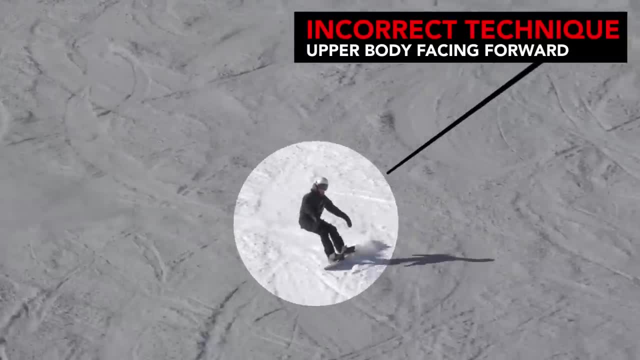 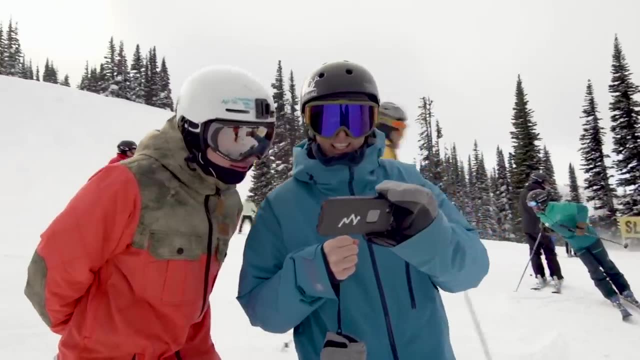 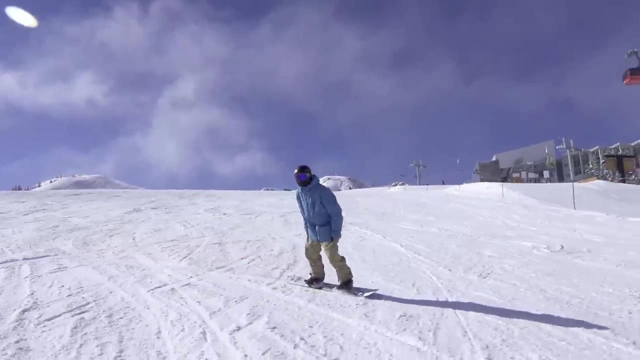 counter-rotate your turns or ride forward until you get to see your own riding on video. If you do, you're going to want to break this habit. to increase the stability of your riding, Try grabbing your pants while practicing some turns. This will aid as a subtle reminder to 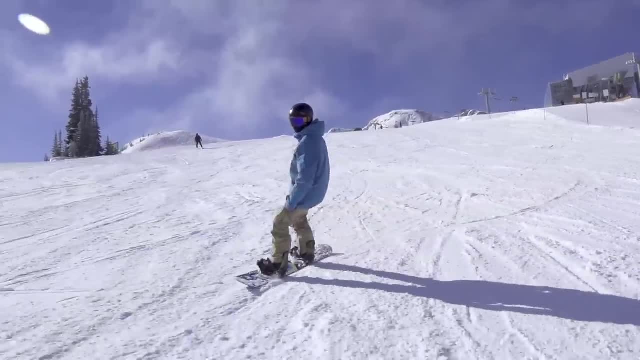 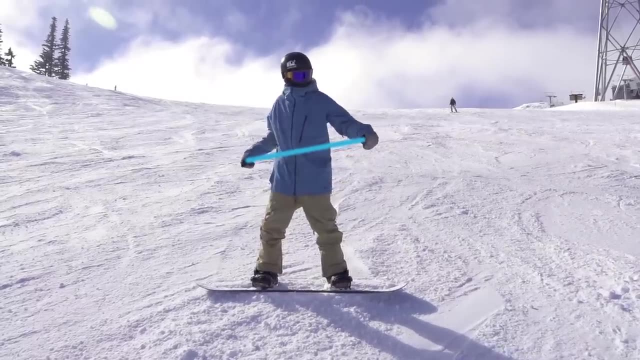 keep your upper body and lower body moving together in the same direction through each turn. Imagine you have a pole that goes through your body and you're holding on to the end of each pole To turn your snowboard. turn the pole through your hips.